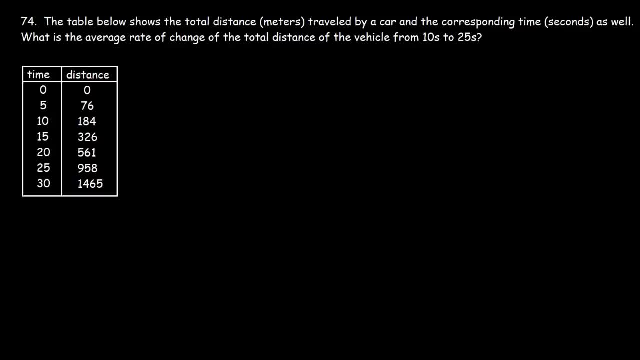 total distance of the vehicle from 10 seconds to 25 seconds. So, based on the last example, go ahead and try this problem. So the average rate of change is going to be the distance, or the change in distance divided by the change in time. So we want to find the answer from 10 seconds to 25 seconds. 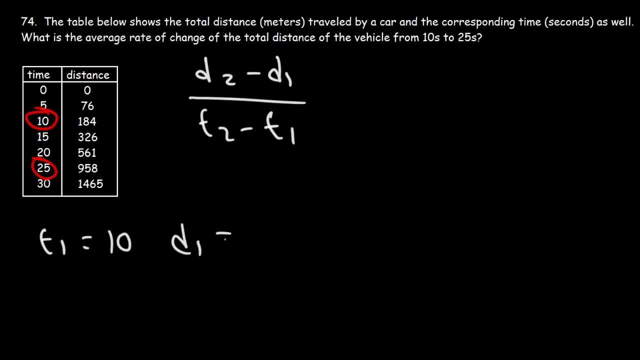 So T1 is going to be 10.. D1, the distance that corresponds to that time is 184.. T2 is 25.. So we want to find the answer from 10 seconds to 25 seconds. So we want to find the answer from 10 seconds to 25 seconds. D2 is going to be 958 meters, So let's plug in what we have right now. So let's replace D2 with 958,, D1 with 184,, T2 with 25, and T1 with 10.. 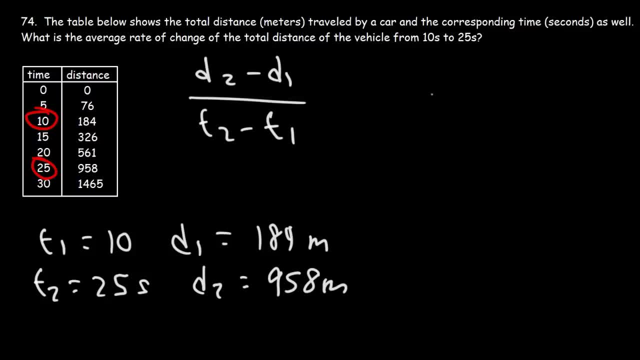 958 minus 184, that's going to be 775.. So we want to find the answer from 10 seconds to 25 seconds, So let's plug in what we have right now. So let's replace D2 with 958, D1 with 184,, T2 with 25, and T1 with 10.. 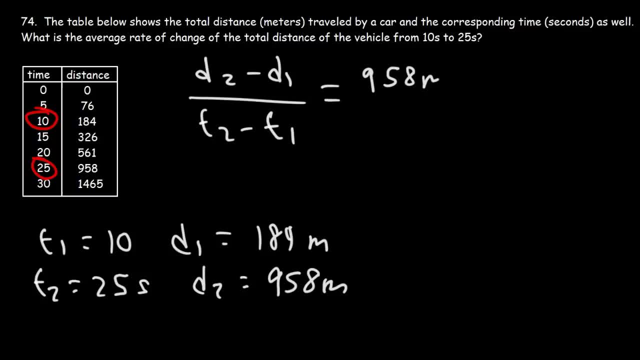 So let's replace D2 with 958, D1 with 184,, T2 with 25, and T1 with 10.. you place D2 with 958, D1 with 184, T2 with 25, and T1 with 10.. 958 minus 184, that's going to be 774.. 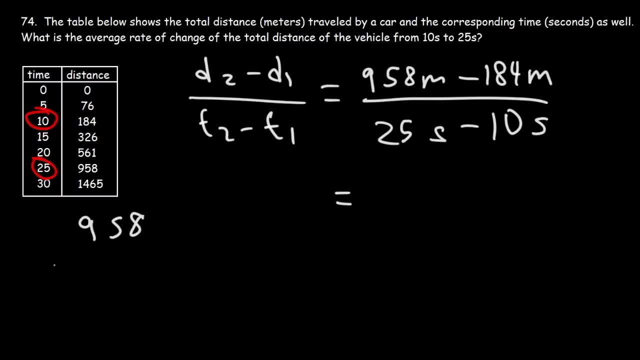 Now let's say, if it's not a calculated problem, here's what you can do to subtract it. So 8 minus 4 is 4.. We can't do 5 minus 8, because that's going to give us a negative number. 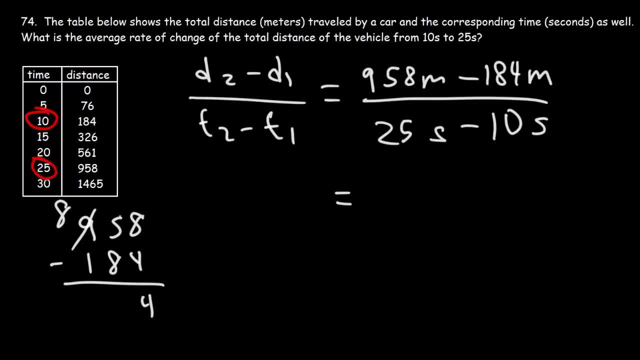 so we need to borrow a 1 from 9.. Turning that to 8,, 5 becomes 15.. 15 minus 8 is 7, and 8 minus 1 is 7.. So we get 774.. 25 minus 10 is 15.. Now I'm going to use the calculator for. 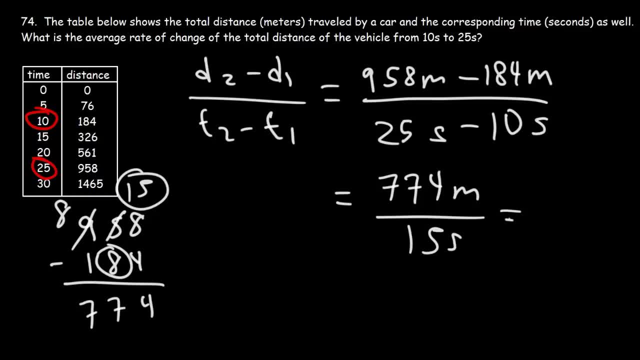 this part. You could use long division if you want to. 774 divided by 15, is 51.6.. Now the units. what do you think the units is going to be? So? notice that we're dividing meters by seconds, So this is going to be meters per second. 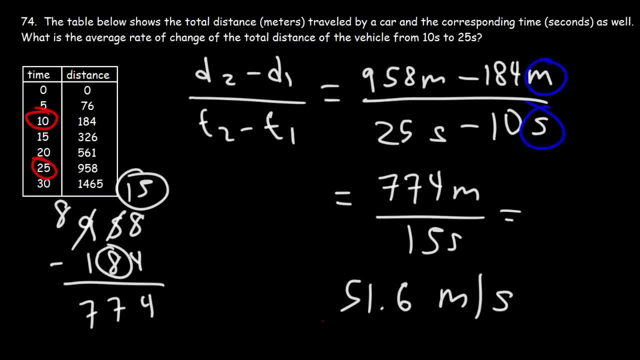 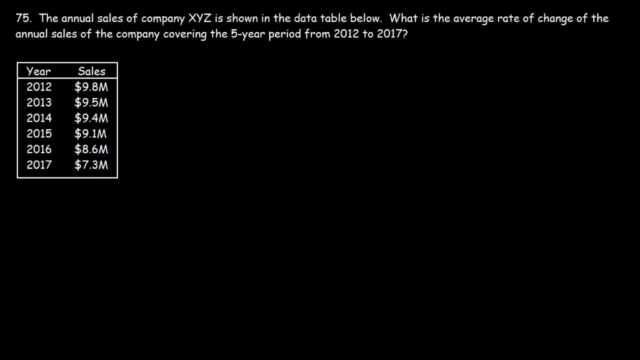 The average rate of change of distance with respect to time is speed. Let's work on one more problem similar to the last one. So we have the annual sales of company XYZ and we have the units. So we're going to divide the annual sales of company XYZ by seconds. 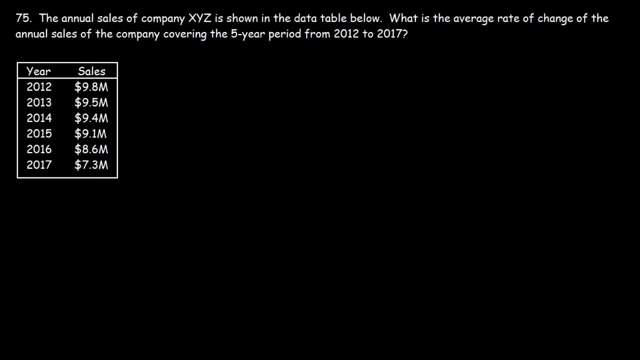 So we have the annual sales of company XYZ and we have the units, So we're going to divide the year that corresponds to those sales. What is the average rate of change of the annual sales of the company covering the five-year period from 2012 to 2017?? So what we're going to do is take. 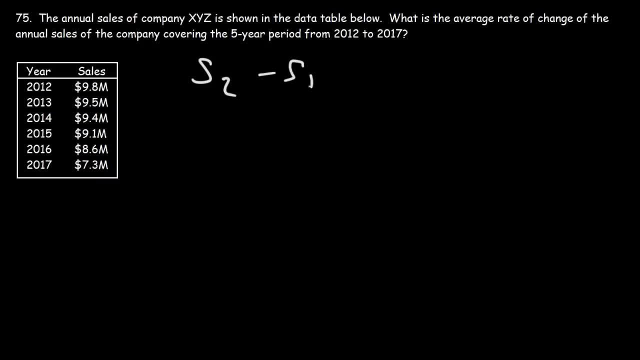 the sales at, let's say, a second point, minus the sales at the first point and subtract it by T2 and T1.. So the first point is at 2012.. So we're going to divide the annual sales of the company XYZ by 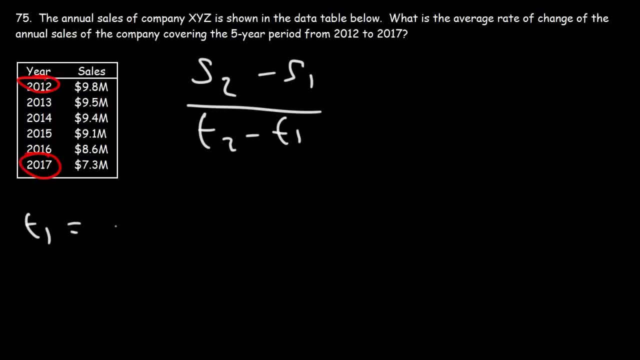 seconds. So we're going to divide the annual sales of the company XYZ by 12.. The second point is 2017.. So our T1 value is 2012.. Our S1 value is the sales during that year. That's 9.8 million. 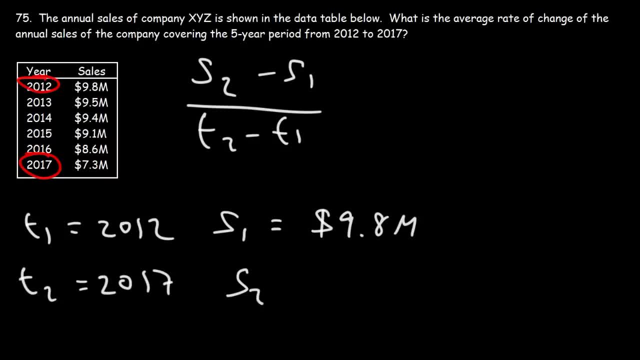 T2 is 2017, and the sales for that year is 7.3 million. So let's plug in what we have: S2 is 7.3 million. S1 is 9.8 million. T2 is 2017 minus T1.. 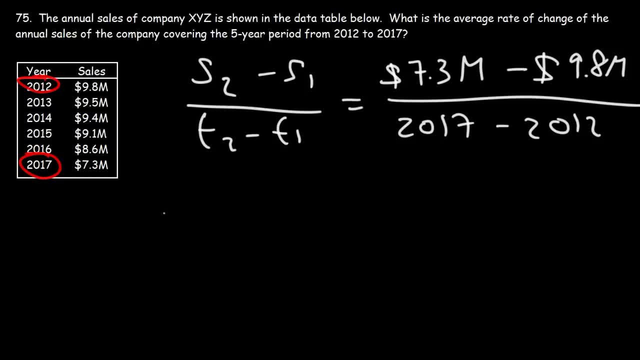 7 minus 3 is negative. 2. 8 minus 3 is 5.. So 7.3 minus 9.8, that's going to be 2.5.. So over the five-year period the annual sales dropped by 2.5 million. 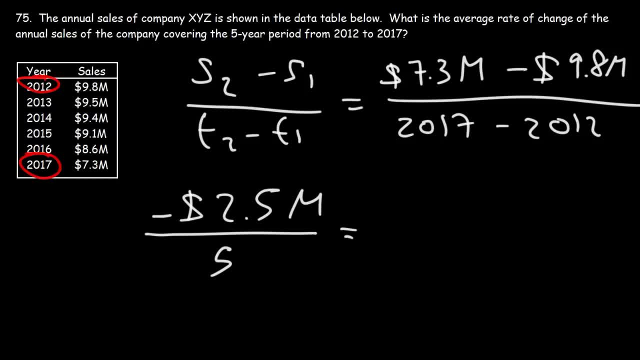 17 minus 12 is 5.. now, what is 2.5 divided by 5? we know that 25 divided by 5 is 5, so 2.5 divided by 5 is 0.5. if you break down 2.5 into 5, equal point. i mean not points, but if you break down 2.5 into 5, equal. 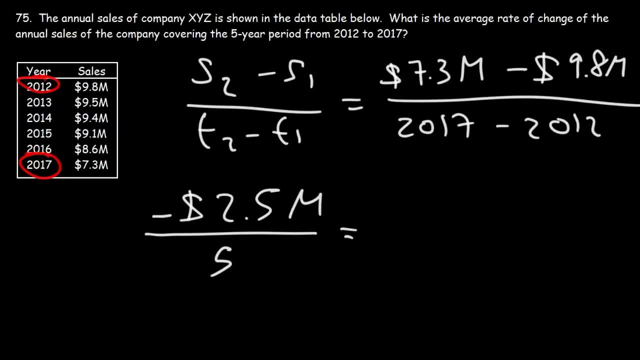 parts. that's what i meant to say. you're going to get 0.5. so the average rate of change in the annual sales of the company per year is negative 0.5 million. so on average, every year the annual sales is decreasing by half a million or 500,000. 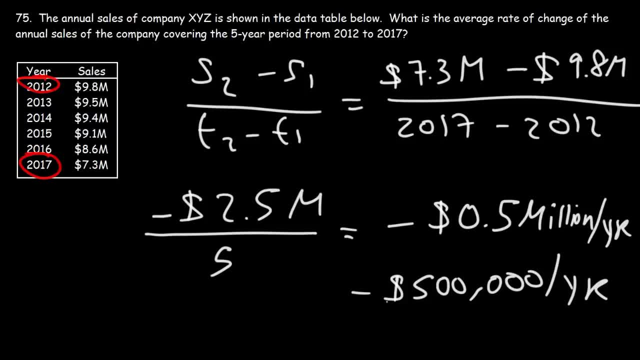 so you don't want to buy the stock in this company. they're not doing too well. so now you know how to calculate the average rate of change of something. so that's it for this video. thanks for watching.